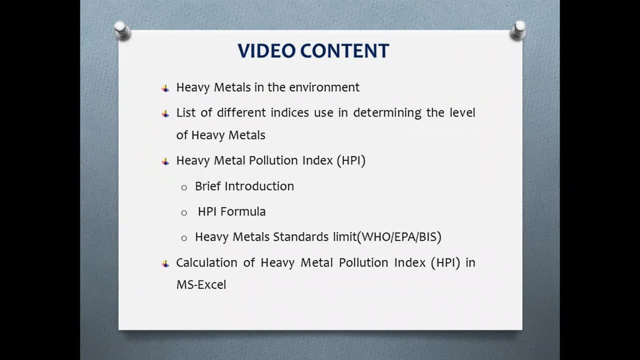 following sections: First, we will talk about the general concept of heavy metals in the environment, and there are different types of index method developed by different researchers for determining the level of heavy metals in the environment, such as soil, sediment, water samples, etc. An HPI is one among those index methods, and after which we 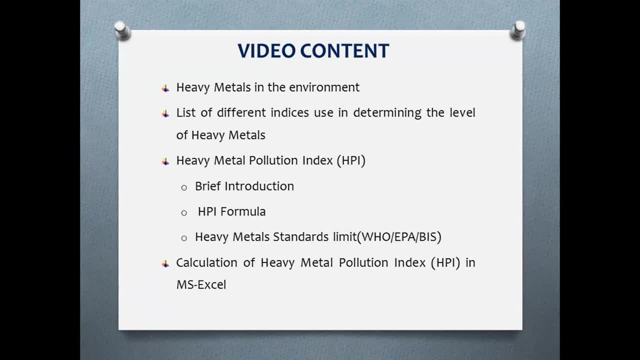 will then dive deeper into the topic, that is, the heavy metal pollution index. First we will see who developed the HPI method and then what it is used for. Then next, we will see the formula used for HPI calculation. Then we will see the tabular representations of the values of 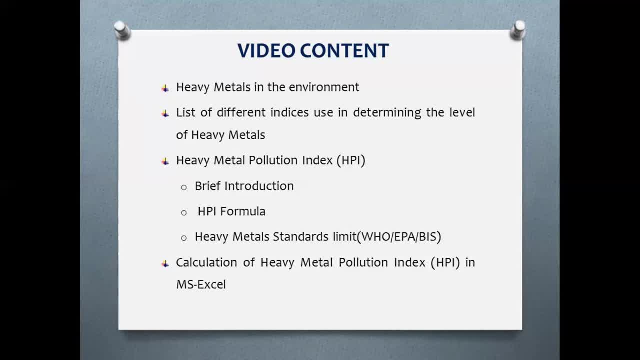 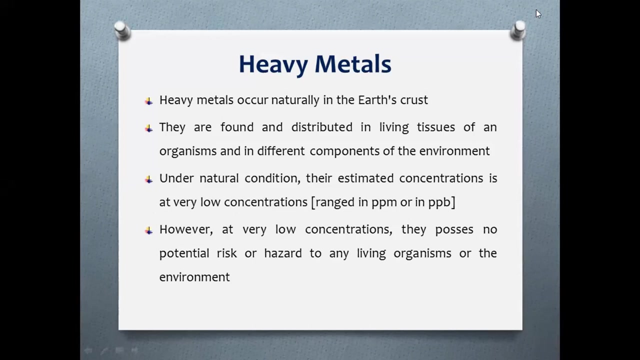 the different heavy metals and their respective standard limits and desirable limits, as described by different recommended agencies such as WHO, EPA and BIS. And, at last, I'll demonstrate to you the hands-on calculation of HPI using Microsoft Excel. To begin with, first of all, let 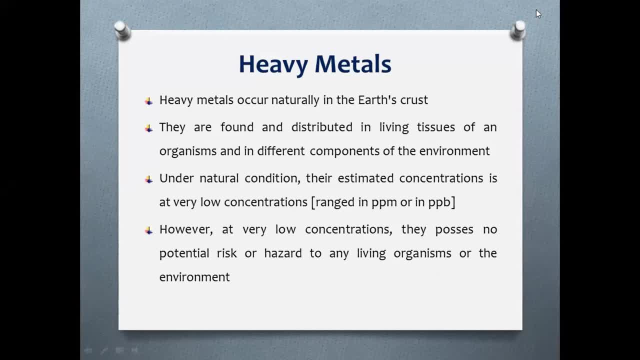 us briefly try to understand what are heavy metals in the environment. Heavy metals are the naturally occurring elements found in the earth crust. Due to this, heavy metals are found to distribute in different living tissues of an organism and also in various components of the environment. However, under natural condition, their concentration. 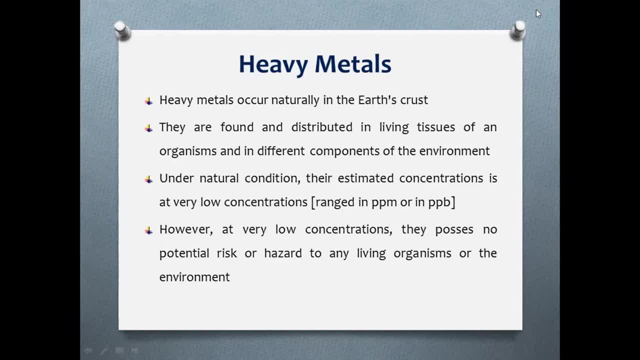 or level is estimated to be very low or insignificant, with values ranging in parts per million or in parts per billion. Therefore, at such a low level or concentration, the heavy metals have no significant health impact or pose no potential health risk to any living organisms. 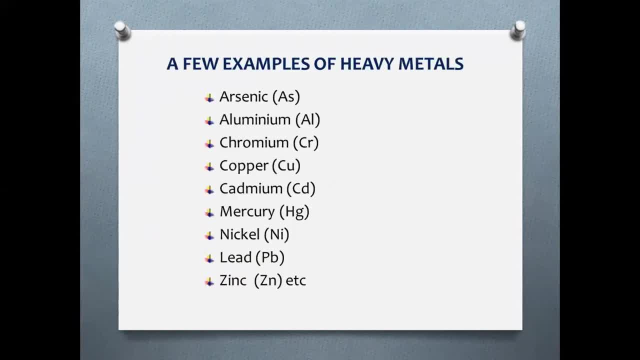 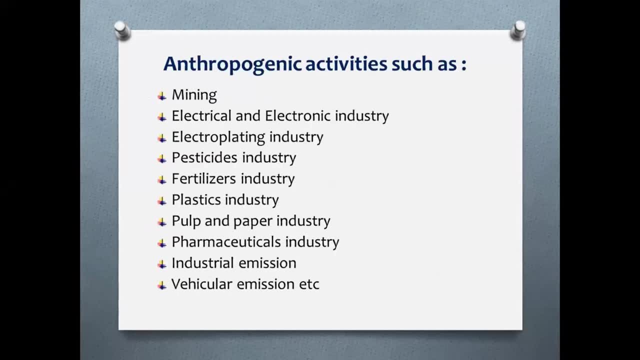 or the environment. Few examples of heavy metals are arsenic, aluminum, chromium, copper, cadmium, mercury, nickel, lead and zinc. On the contrary, with modernization, industrialization and advancement of human civilization over the past decades, various anthropogenic activities such as 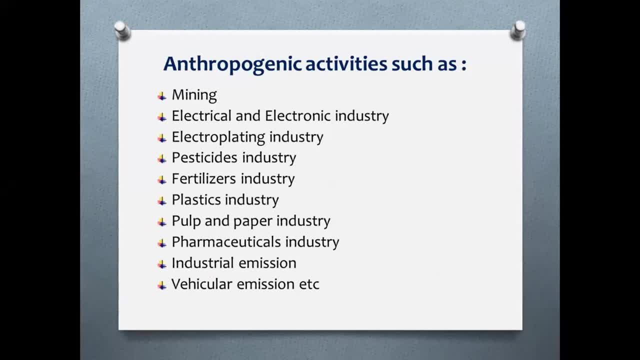 mining and the presence of electrical and electronic industries, electroplating industries, pesticides industries, fertilizers industries, plastic industries, pulp and paper, pharmaceutical industries, industrial emissions, vehicular emissions, to name a few. These activities are known to release quantum amounts of various pollutants, including heavy metals, into the. 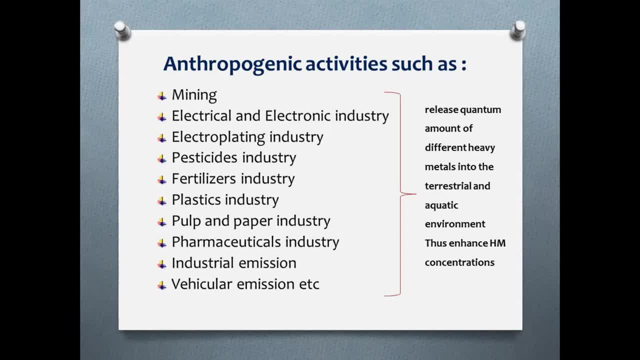 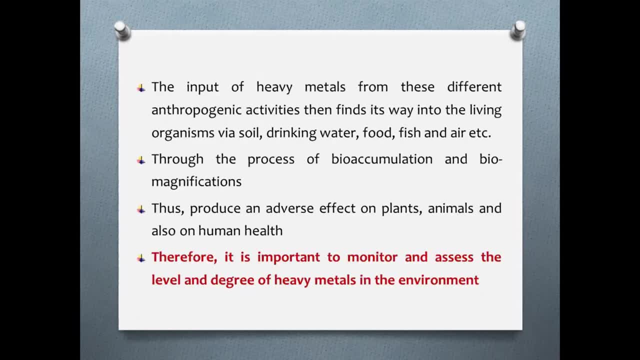 different components of the terrestrial as well as the natural environment, Thus resulting into the exponential rise of heavy metals level in the environment. Now, when in the environment, these heavy metals later find their ways into the living organism through soil, drinking water, food, fish, air, etc. And through the process of bioaccumulation? 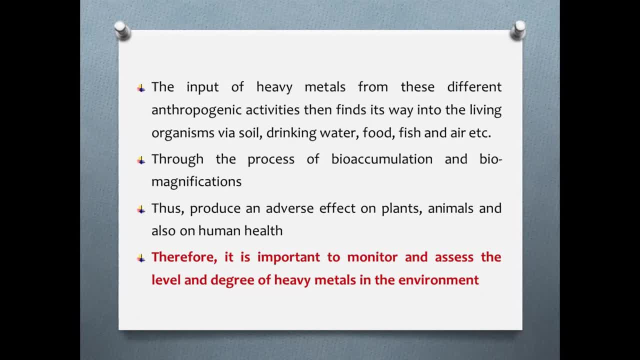 and biomagnification. these heavy metals are found to produce an adverse effect on plant animals and even on human health. So with this basic explanation we now we can conclude that it is vital to monitor and assess the level and the degree of heavy metals in the environment. 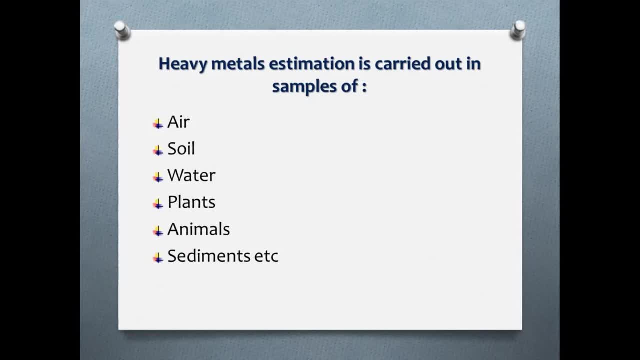 Generally, concentration of heavy metals is estimated or studies in sample of air, soil, water, plants, animals, sediments, etc. And for studying these the analytical methods and estimation techniques adopted are totally distinct and different from one another. For example, soil analytical method and estimation techniques. 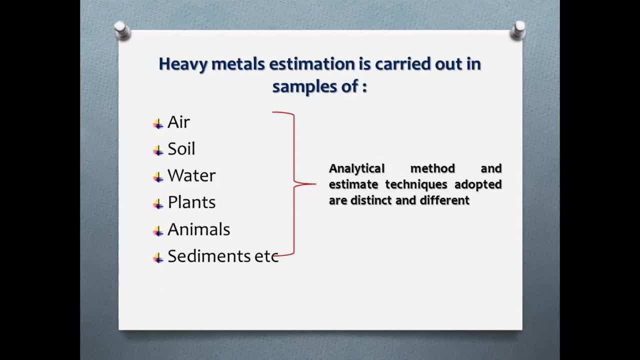 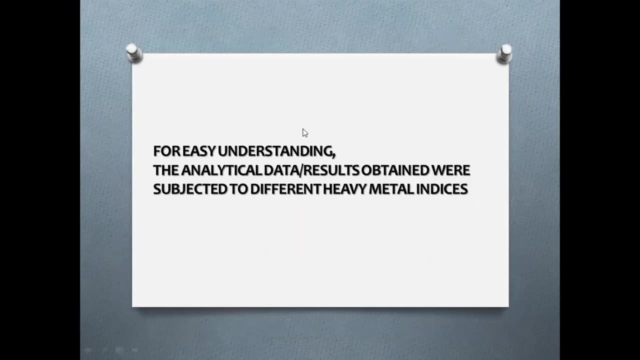 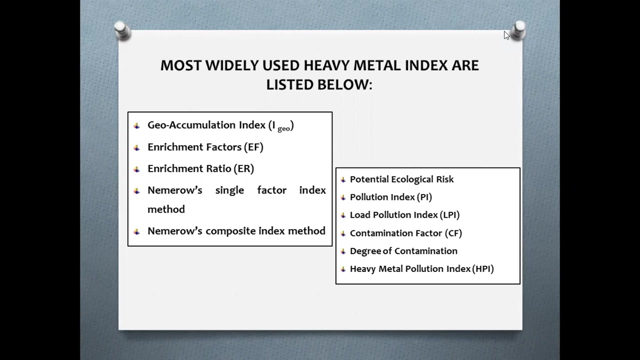 is totally different from that of the sediment uh analytical method and estimation techniques. However, after analysis, for easy understanding, the analytical data or results obtained are subjected to different heavy metals indices of choices. These are the list of different widely known heavy metal index method which have been used by different researchers In one of my video. 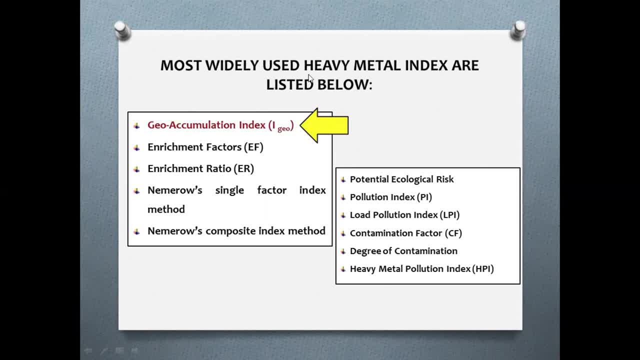 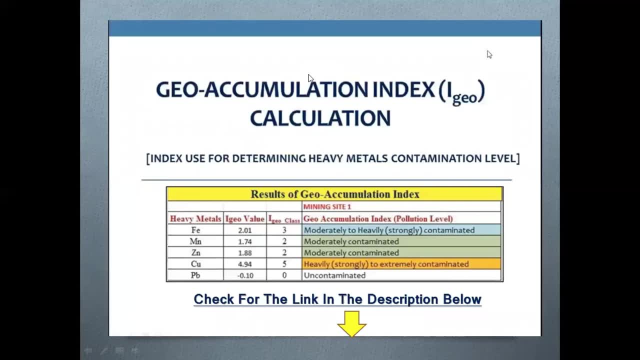 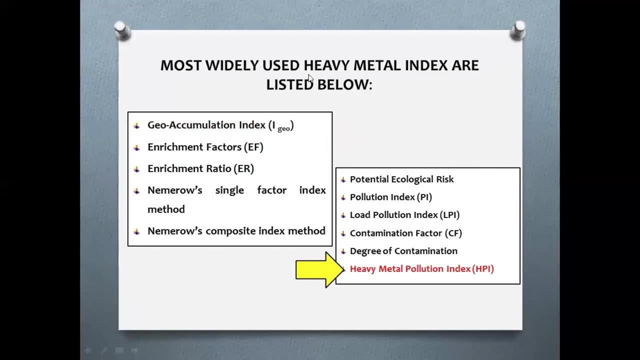 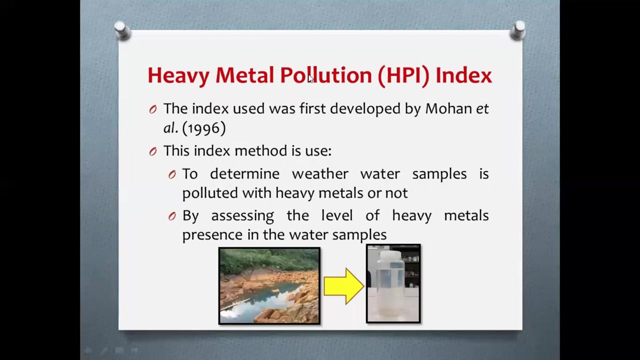 uploaded earlier I shared about geoaccumulation index. If you are interested in geoaccumulation index method, you can check the link in the description given below or in my channel. In this video we'll be learning about heavy metal pollution index, or HBI. This index method was developed by Mohan et. 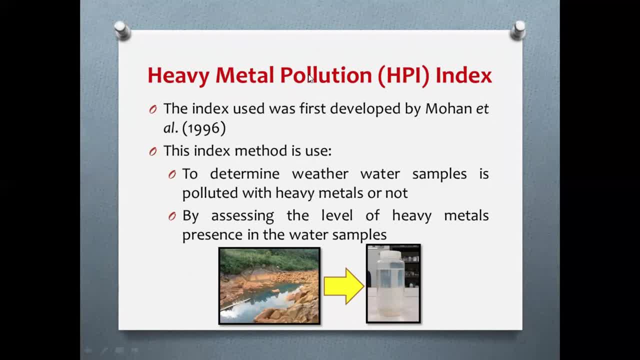 al in the year 1996.. The main objective of this index method, right from the time this index method was developed, was to reduce the amount of heavy metals that are produced in the environment. The main objective of this index method, right from the time this index method was developed, was to reduce the amount of heavy metals that are produced in the environment. 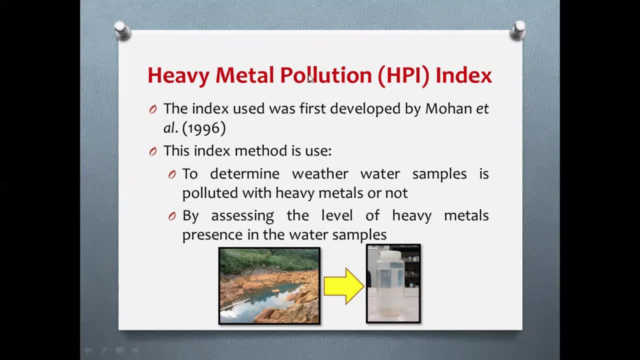 To determine or find out whether any water samples of interest is contaminated or polluted with heavy metals or not. So how to determine or find this out? Simply, this can be done by analyzing the collected water samples using Atomic Absorption Spectrophotometer, or AAS. 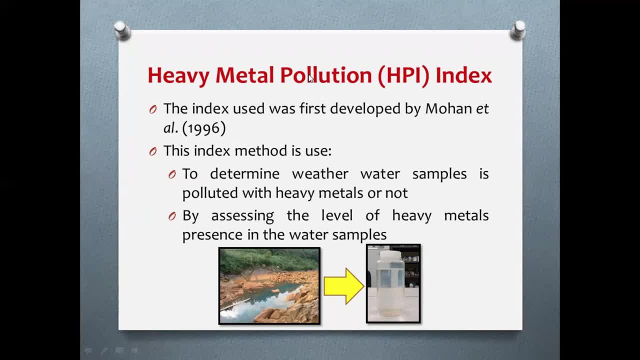 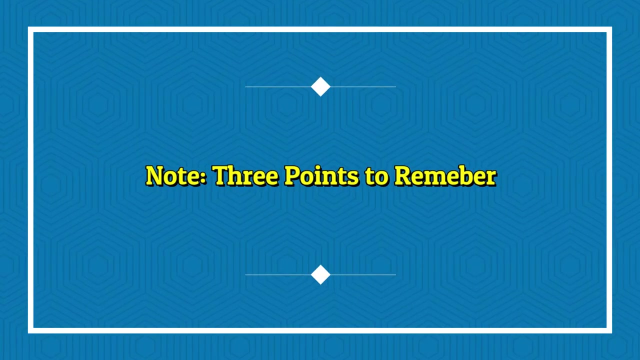 Then the analytical results obtained will be subjected to HPAI calculation, and after which you will then obtain an HPAI value, and that HPAI value will ultimately provide you information whether the water samples being analyzed is contaminated with heavy metals or not. For this index method, there are three important points one needs to remember. 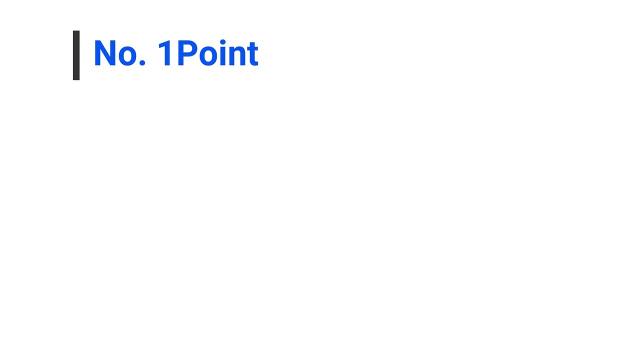 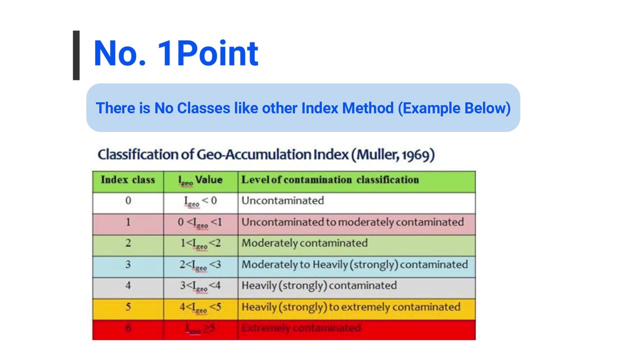 The number one point to remember is this index method is unlike other heavy metal index methods where the calculated index value will fall under any of the different classes or range, which then represents HPAI, The level of heavy metals present in the samples of interest. 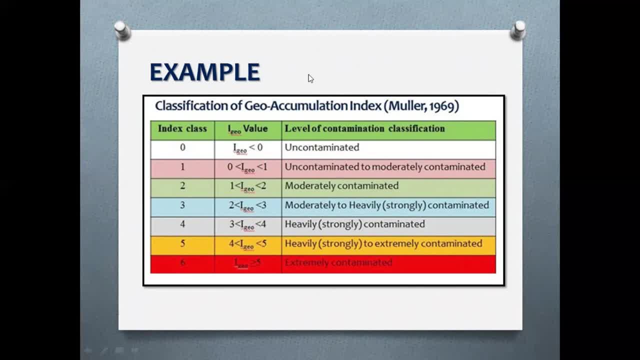 For example, in the Geoaccumulation Index, the calculated HPAI will be based on the calculated value obtained. Then we can determine the classes, which classes we belong to and from the class we will then be able to determine the level of contamination. 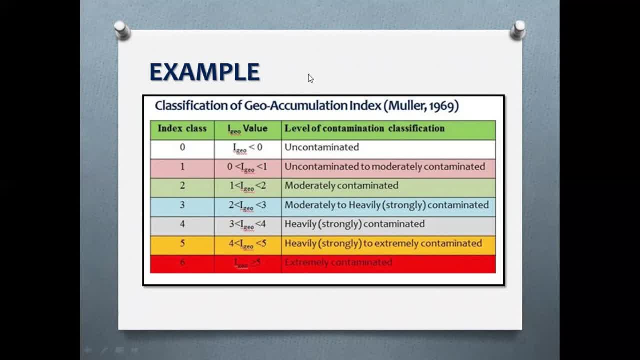 So basically, for example in the Geoaccumulation Index, when we say the index class belongs to class 1, it means that the sample is uncontaminated to moderately contaminated. If we say that the index class falls under class 6, then we say that the sample is. 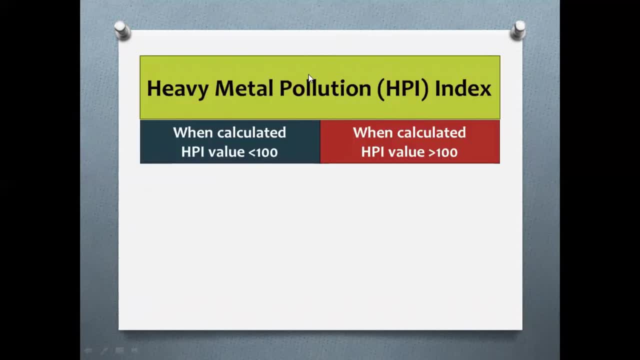 extremely contaminated with heavy metals. But for this particular index method, remember that once the calculation of HPI value is completed, remember that the HPI value you will obtain will be either above 100 or below 100. That is, when the HPI value is less than 100, it indicates that 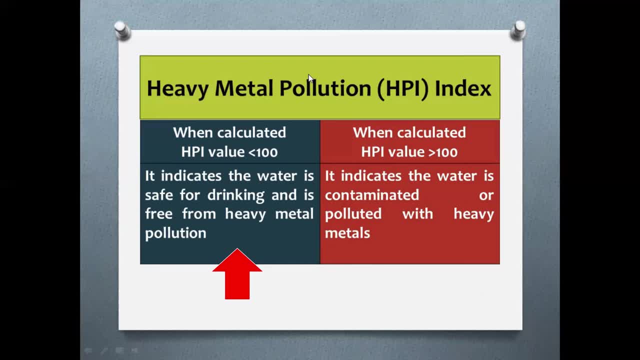 the water sample is safe for drinking and is free from heavy metal pollution, because the HPI value for permissible or critical pollution index for drinking water is 100. But if the HPI value you obtain is greater than 100, then it indicates that the water 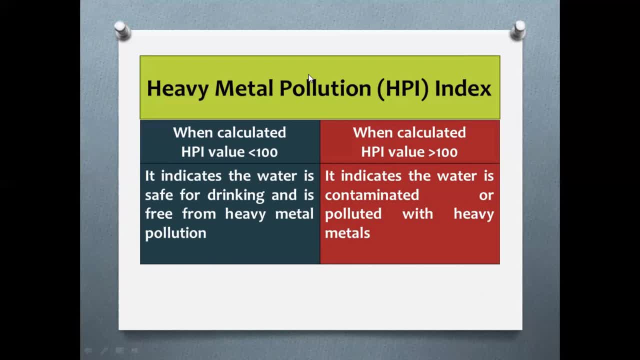 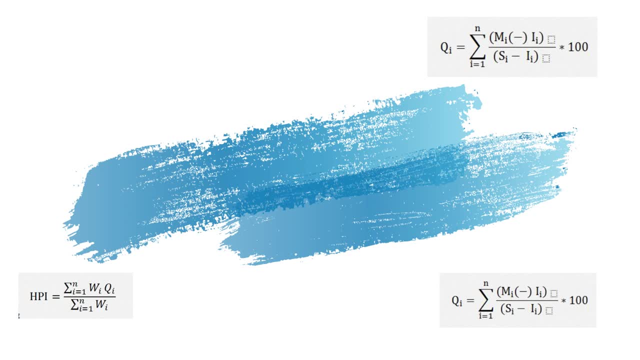 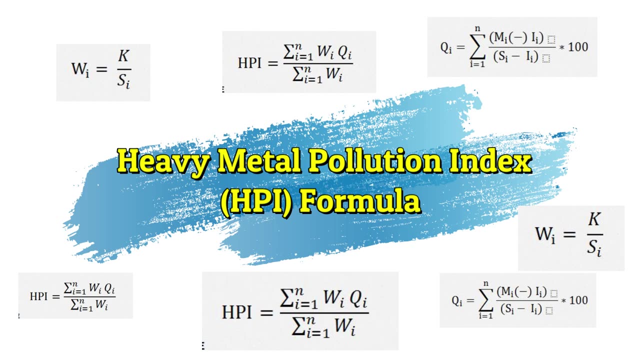 sample is contaminated or polluted with heavy metals. Now, once you are clear with the basic introduction and important information on HPI, we will now move on to the next part of the topic, that is, the heavy metal pollution index formula. But before we move into the formula of HPI, you need to know that the HPI formula consists of two. 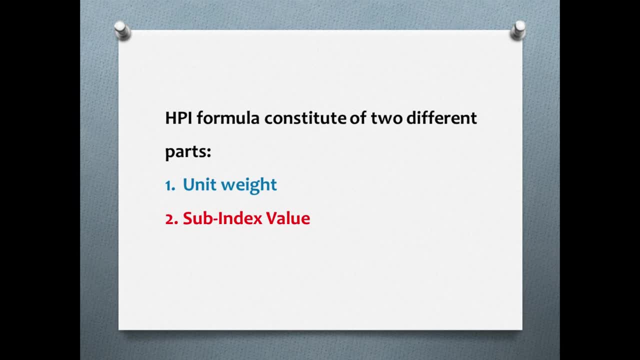 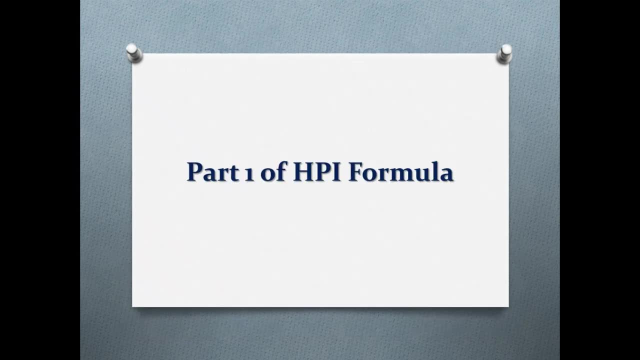 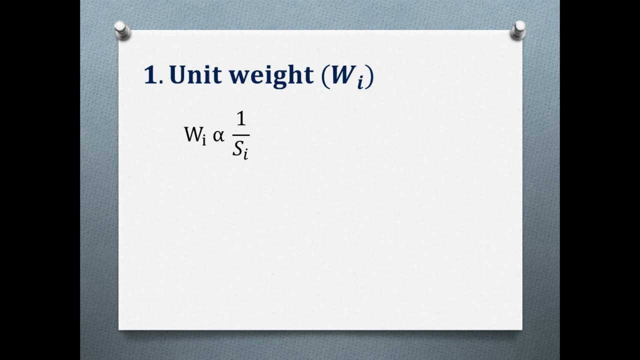 different parts. The first part is on unit weight and the second part is the sub-index value. So first let's see the first part of the HPI formula, which is the unit weight or the WI value, since in normal numbers unit weight is inversely proportional to SI, or WOI is equal to K divided. 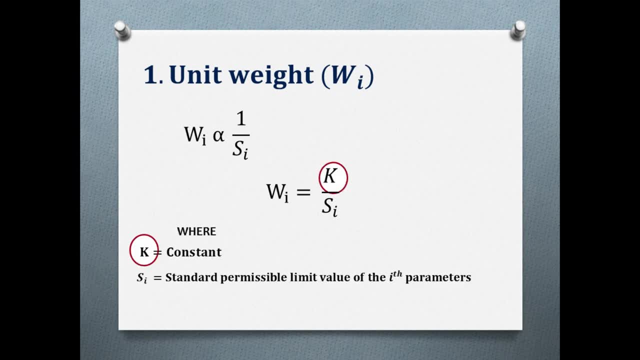 be SI, Where K stands for constant or, if you see, in most of the research paper for this particular heavy metal index method we already said K-value and KI value are same but cualiterized to K-value, medias value is given as 1 or unity and where SI stands for the standard permissible. 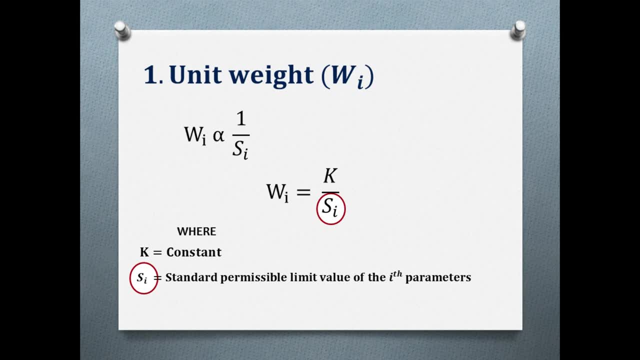 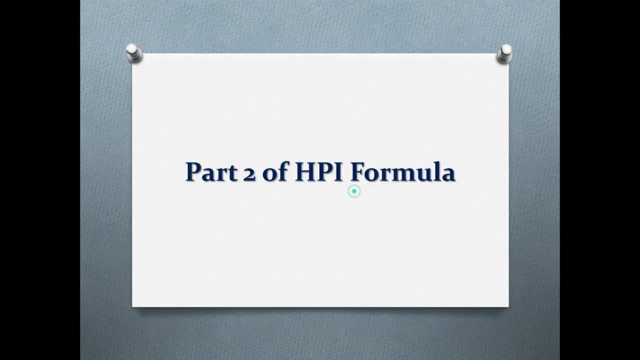 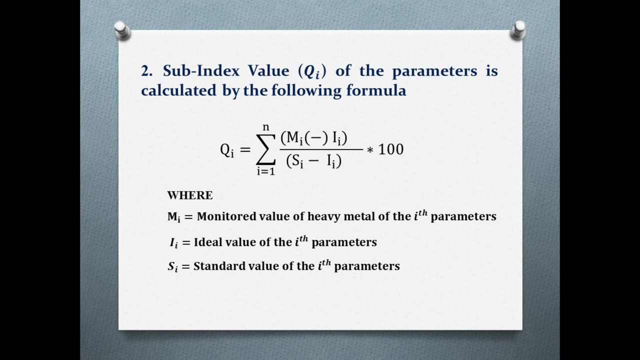 limit of the ith parameters. so which means that using this formula, we will be calculating for the WI value. okay, and similarly we'll see for the second part of the formula, which is the subindex value, or the QI value. QI value is given as summation of MI minus II divided by SI minus II in 200: the same formula. 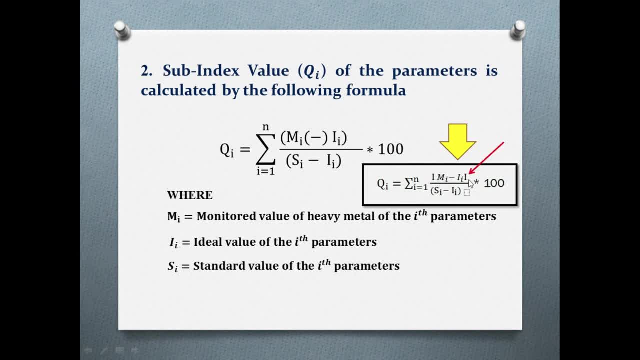 sometimes. you'll see it is in this format, with only differences. you'll see in this part where they give: here is the modulus sign. what does it indicate when you have this or when you have this? basically, any negative values can be ignored for the calculation part. all right, now let's see in detail about this. 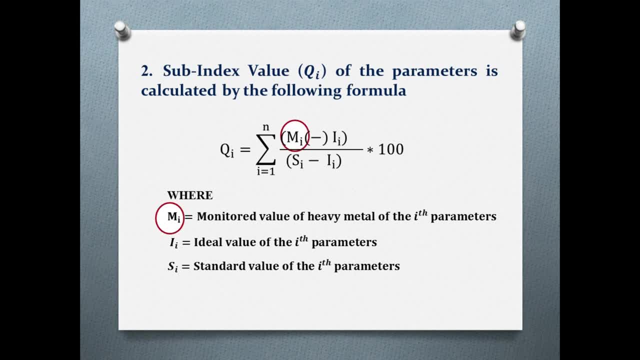 subindex value, or the QI. here, MI stands for the monitor value of heavy metals of the ith parameters, which means that is the value that you obtain during the analysis of your sample. that will be your monitor value, and II stands for the ideal value of the ith parameters and SI is the standard value of the ith. 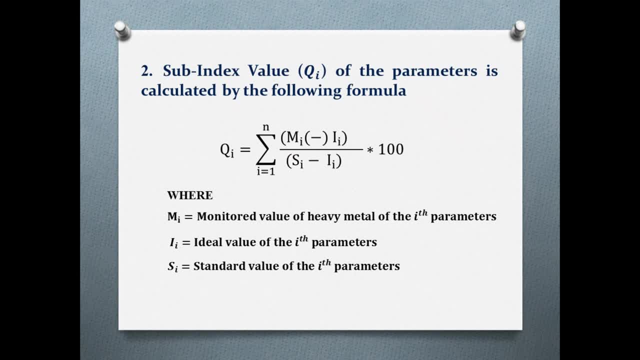 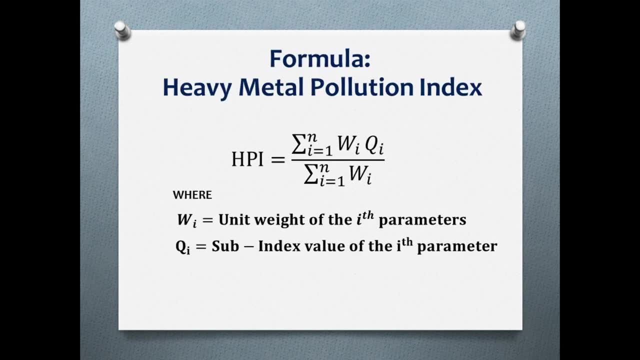 parameters. now, merging the WI and QI formula together, the HPI formula is obtained, and this is the HPI formula. now, using this formula, calculation of the HPI value for any heavy metals of interest in what a samples can be carried out, and the HPI formula is given, as HPI is equal to summation of. 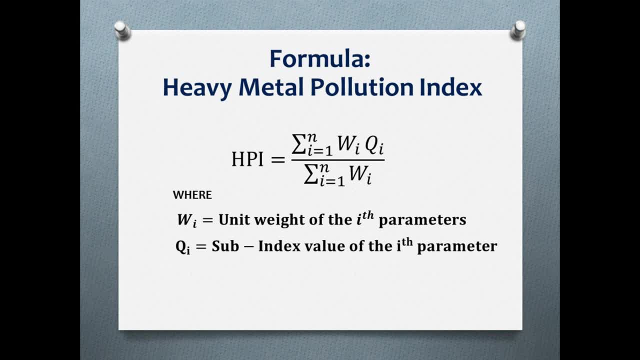 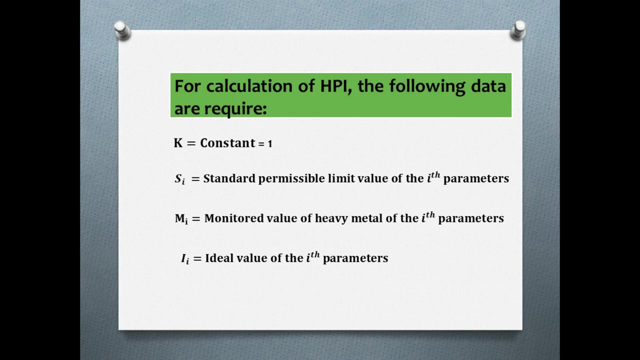 WI by Qi, divided by summation of w of I, where wi stands for the unit weight of the i-th parameters and qi is the sub index value of the i-th parameters. now, from this formula we found that for calculation of hpi the following data are required: where k is equal to constant, si is the standard permissible limit of the parameters. 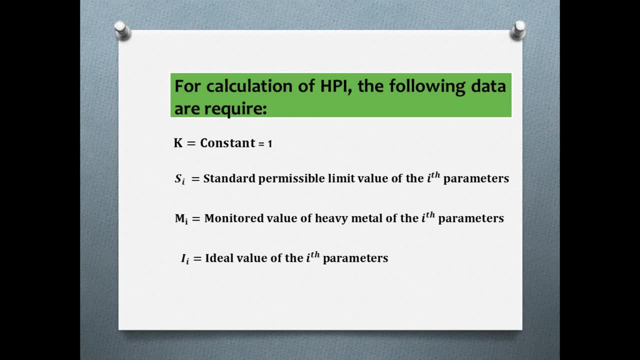 m is the monitor value of the heavy metals, of the i-th parameters, and i is the ideal value of the parameters. if you remember what i just shown you earlier. ki divided by si is the unit weight or the wi right, and if ki is known. but the only thing which is not known to us is the standard permissible. 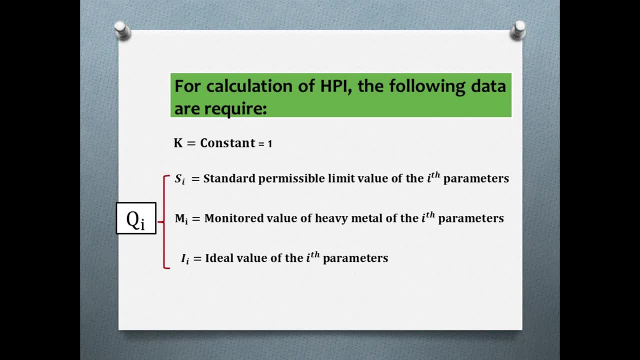 limit of the i-th parameters. similarly, for qi, the data that we require are the si, which is the standard permissible limit of the i-th parameters, mi is the monitor value of the i-th parameters or the analytical data of the i-th parameters. and ii is the ideal. 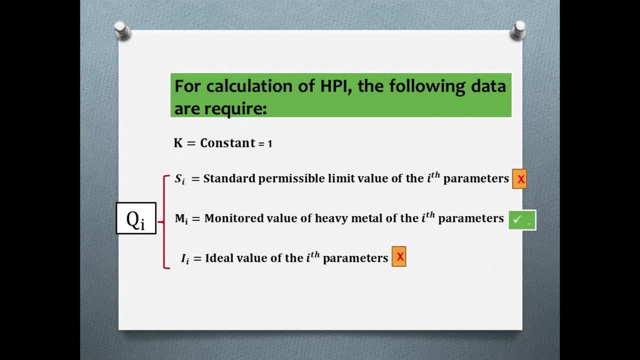 value of the i-th parameters. for qi, we found that si and ii are the things which we don't know as yet, but for mi, once the analysis is done, the analytical data were being obtained. so from here, from where or how do we get the ideal value or the standard limit values, or, in short, the si and the? 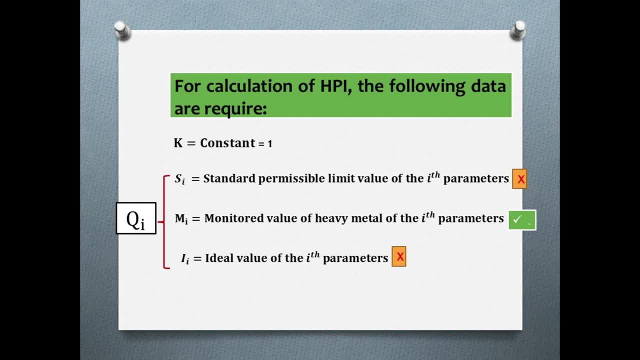 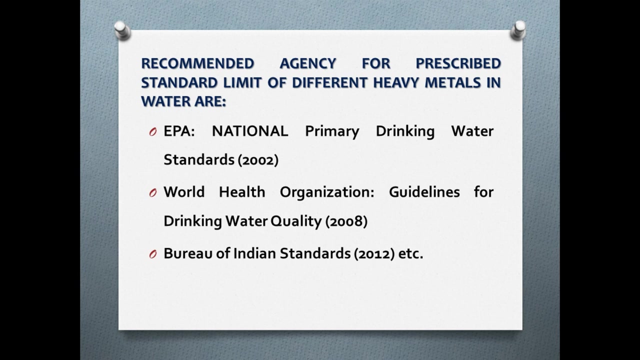 ii values for any heavy metals of interest. the answer is: to obtain the si and the ii value of any heavy metals of interest, we have to refer to the prescribed standard limit developed by different international and national agency, such as the epa who on, or the bis in india. we refer to the 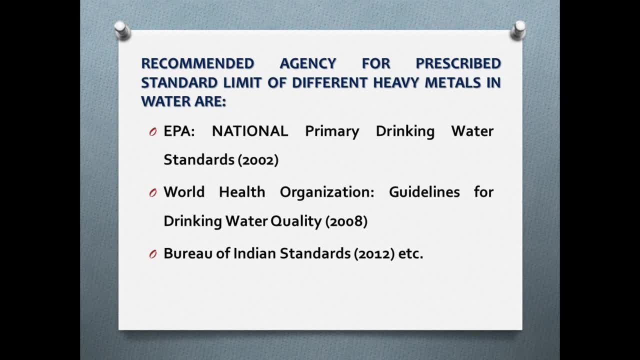 bis acceptable limit and standard limit. similarly, in case if you are not from india, you can refer to your country recommended agency or the epa or the who prescribed limit for different heavy metals in different components of the environment. these different agency that i have mentioned publish the standard prescribed limits. 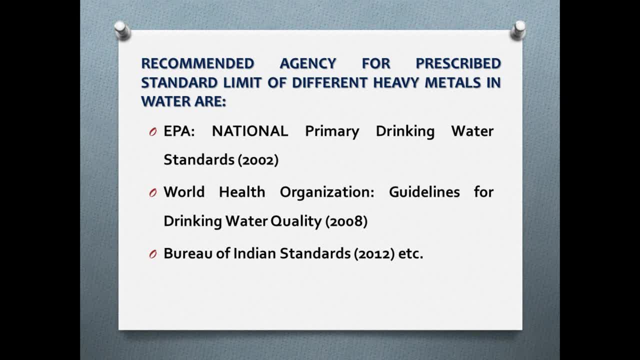 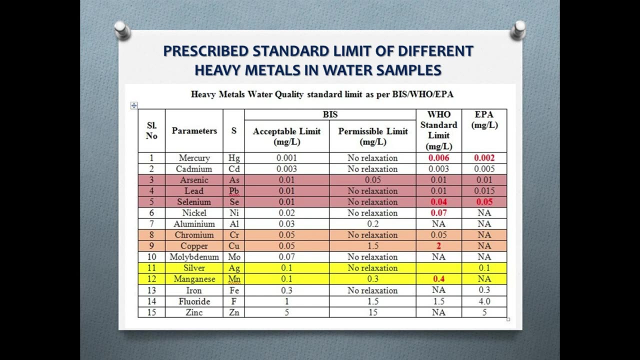 for different environmental parameters, including heavy metals. so from these sources the data for different prescribed limit for different heavy metals in water samples are presented in this table here. in this table you can see that for different heavy metals present in water samples, bureau of indian standards provide both the acceptable limit and the permissible limit. 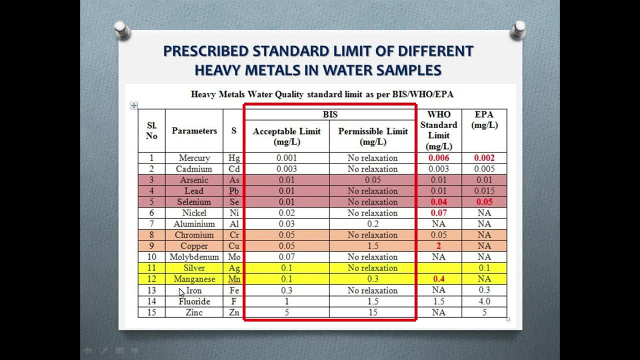 whereas who and epa only provide the standard limit for each heavy metals. keeping this table in mind, the benefit of preparing this table is that it is from this table where you will acquire the si and the ii value. cool, right, but again the next question. sometimes we have to direct. 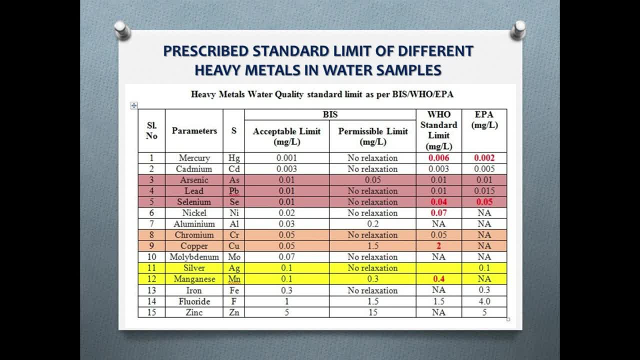 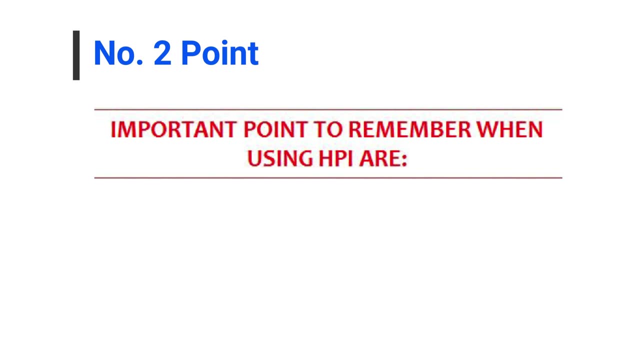 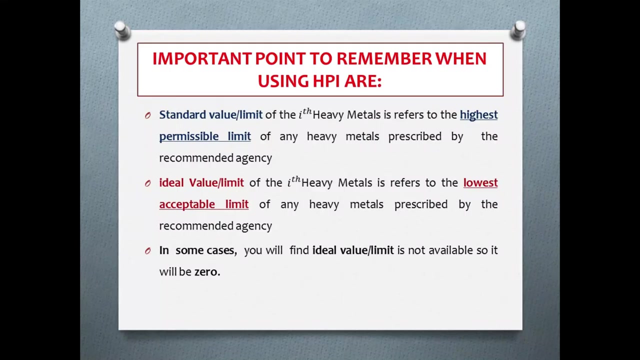 that arises is which values will be for the i-th value and which value will be for SI values. so with this we now come to the point number two, that that a researcher needs to remember when using HPI method of calculation for this index method, when you say standard limit or the SI value of the i-th heavy metals. 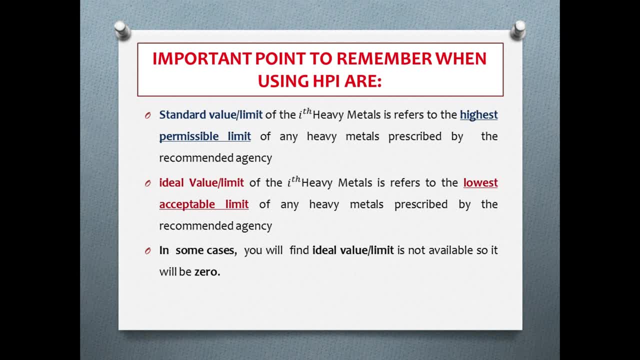 then you are referring to the highest value prescribed by the recommended agency selected for the study. and when you say ideal value or II value of a heavy metal, then you are referring the lowest value prescribed by the recommended agency selected for the study. okay, however, you will come across that in some cases, there will be only 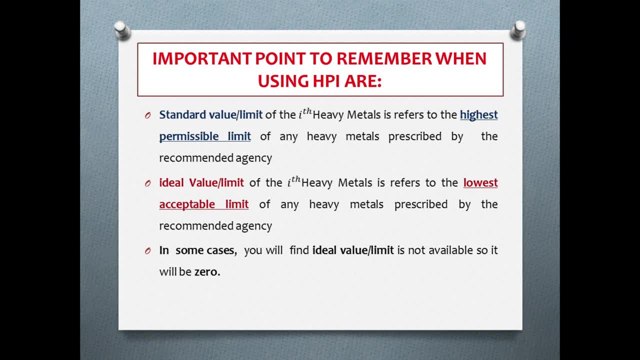 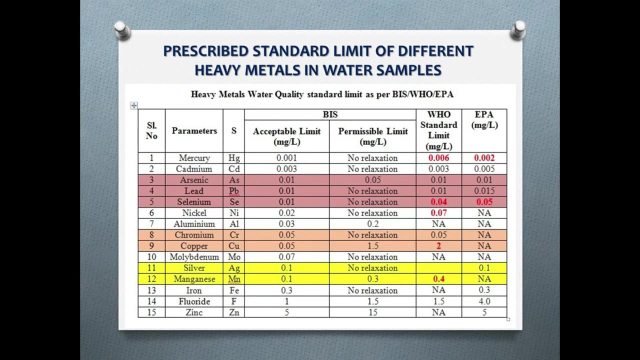 one data for a particular heavy metals. in that case, value will be the SI value and theii value will be zero. now let's go back to that table. okay, so from this table, let's see, let's find out the SI and theii value of, let's say, arsenic. 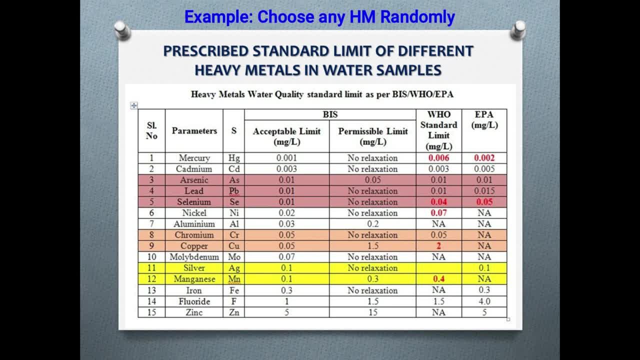 copper, zinc and lead, okay, since for this I'll be using the BIS standards. so from here, for arsenic, you will see arsenic water is arsenic. number three for arsenic snake, you'll have these two values, 0.01 and 0.05, right, so the highest value here will be 0.05. 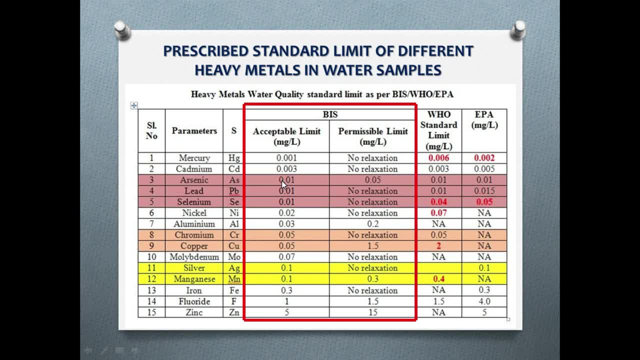 and the lowest value will be 0.01. so your 0.05, which is the highest value, will be your si value and your 0.01 value will be the ii value. similarly, for copper, number nine, you have these two values right: 0.05 and 1.5. now, since this is the lowest value, and 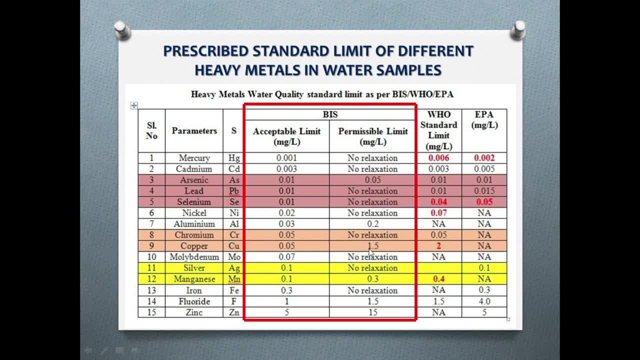 this is the highest value, so i the 1.5 is the highest value, so it will be the si value and 0.05 will be your ii value. similarly, you check for zinc number 15: 5 is the lowest value and 15 is highest value, so the highest value will be the. 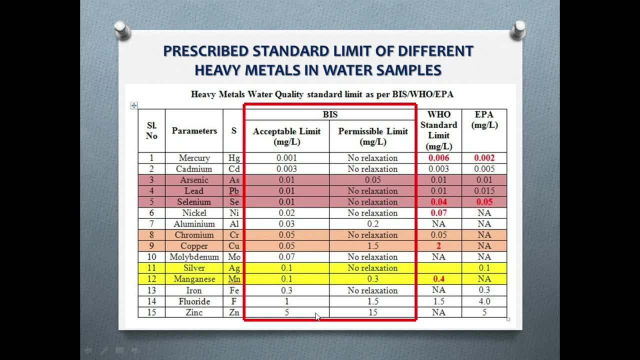 si value and the lower value, lowest value, will be the i i value. and one more, for example lead. now check led. led is number four. now you see that in uh bis the prescribed limit is only acceptable limit, for that is 0.01, and the other value is no relaxation, which means this is only number that is given here. 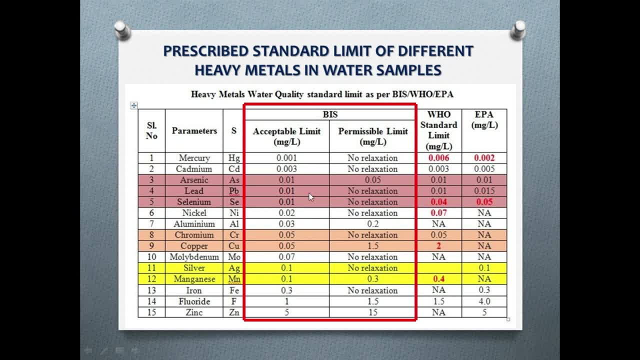 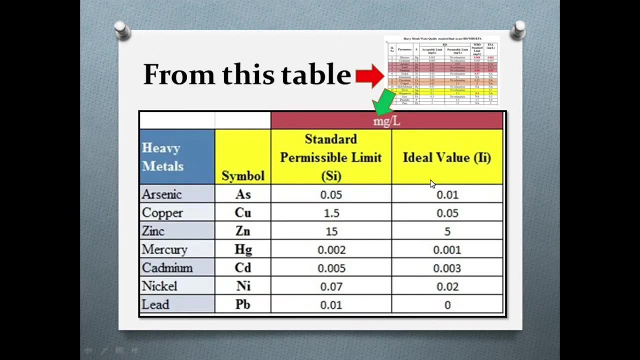 so, which means that for 0.01 will be your si value and since there is, or the value smaller than 0.01, so therefore the ii value for lead will be 0. okay, so, so this is how you will acquire your si and ii value for the heavy metals pollution index. method of calculation. 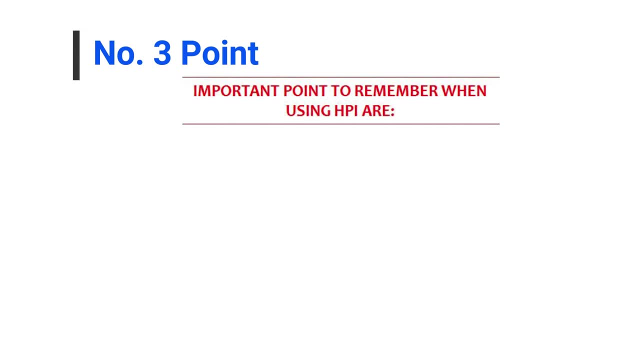 all right. next important point, number three, to remember when, while using the hpi method of calculation, is all analytical data of different heavy metals studied, including the ii value and the si values which are expressed in mg per liter or perth per million, should be converted into. 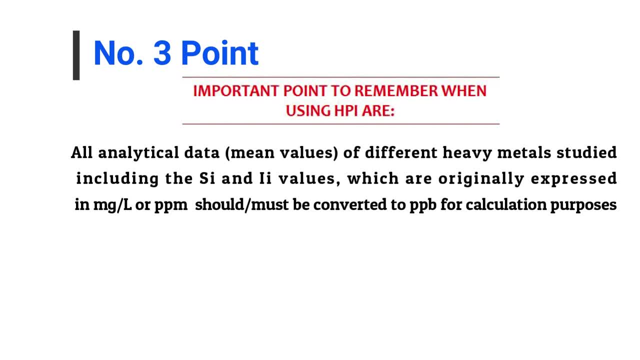 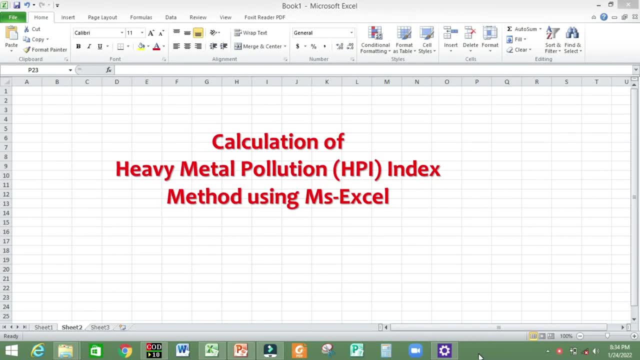 perth, per billion or ppb. this is very important points to remember right. so now, once you are clear about the integral component of the hpi method, the next and the final stage will be the computation of the hpi method using microsoft excel. so, to begin with, for easy understanding of the heavy metal pollution, 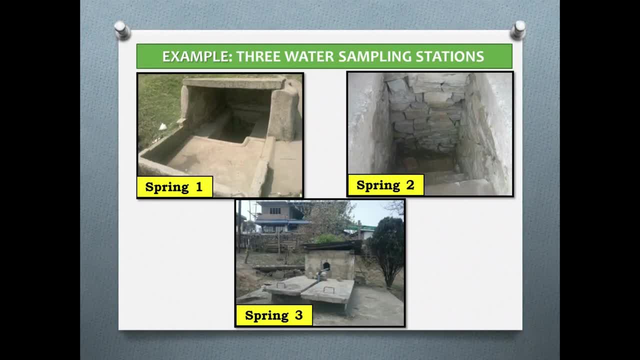 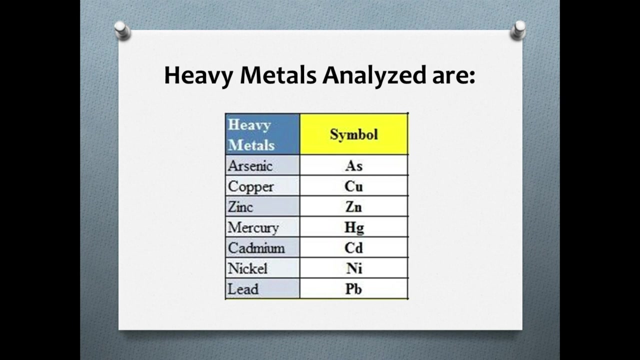 index method. first, let us assume that we are collecting water samples from these three different springs, and the water samples collected were then analyzed for arsenic, copper, zinc, mercury, cadmium, nickel and lead. after analysis, let's assume that the data obtained from the three different sampling stations, or these three, 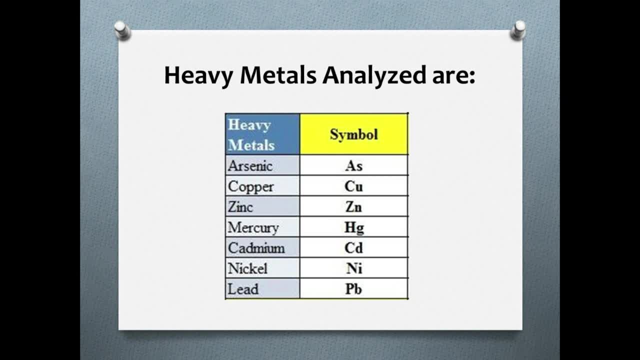 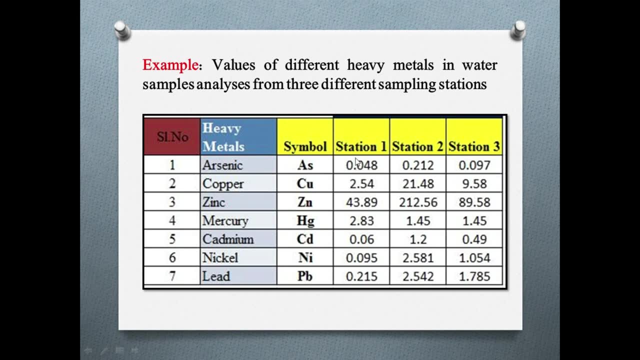 screens for the different heavy metals analyzed are displayed on the screen. so the value for arsenic for station one, or spring one, is this. for station two is this watch. and it's this much. these are all imagined data, okay, just for demonstration purpose. similarly, for this much copper was present. 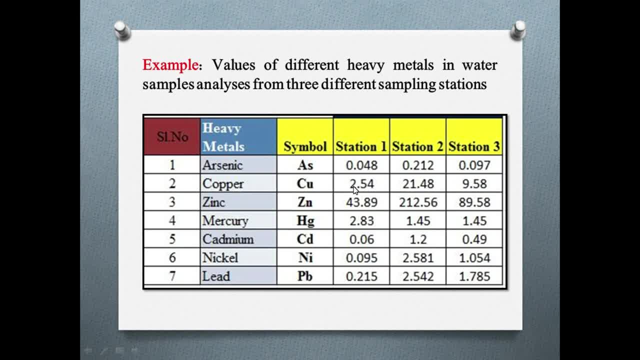 instead in station one or spring one. this much copper is present in spring two and this much copper present spree chaos. similarly, for all onset of rscus perium for response was essentially appearing very then. the method of analysis: Consumption was obtained by ssungs, heavy metals and different respective sampling station. however, for the general 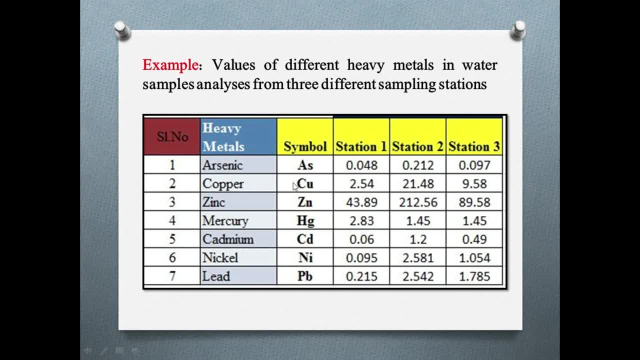 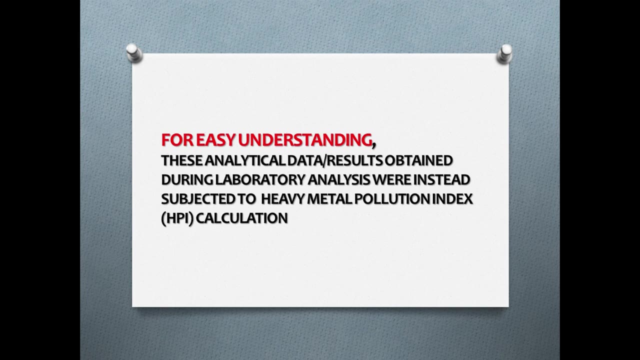 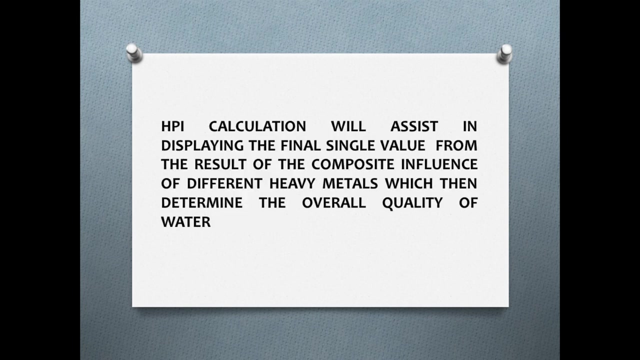 public or the common man, these data might not give a clear indication or information about the level of heavy metals or their overall influence on the water samples studied. therefore, to further simplify these data and also to interpret the results easily, the data obtained during laboratory analysis were instead subjected to HPI calculation, and the output of the calculation will give: 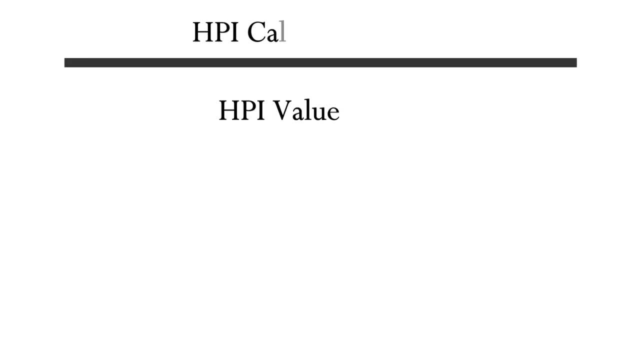 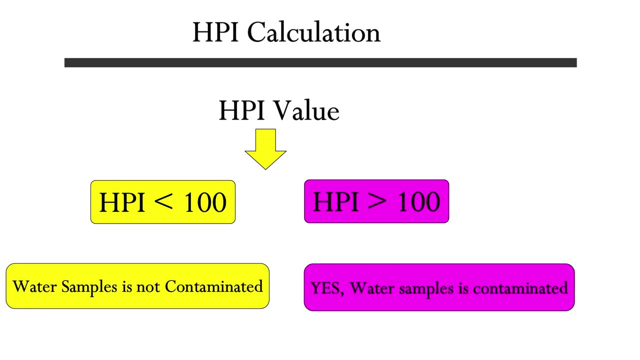 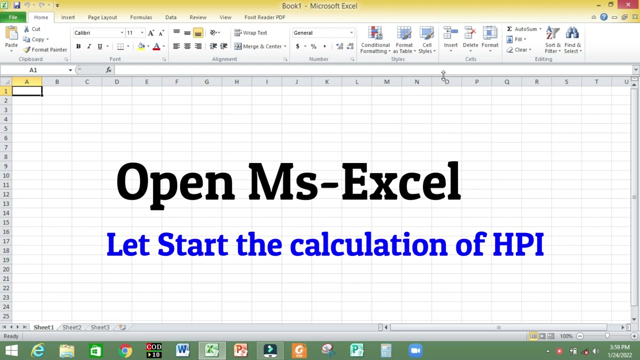 us a single value that is either less than 100 or above 100, and this will reflect the results and specifically provide information to us whether the samples is contaminated with heavy metals or not. next let's open MS Excel sheet and, for demonstration purposes, let's assume that 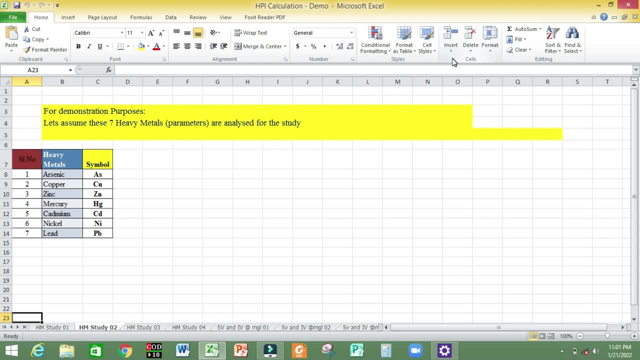 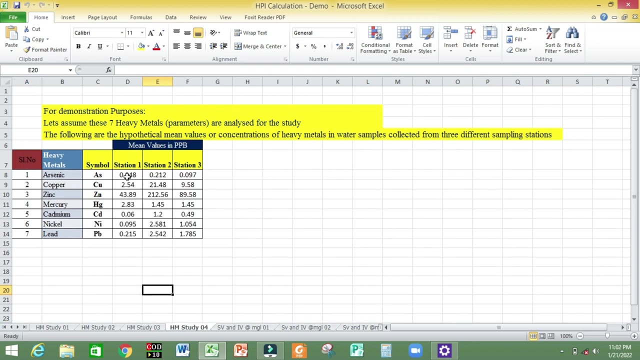 in our hypothetical study, heavy metals are analyzed in the water samples- that are arsenic, copper, zinc, mercury, cadmium, nickel and lead. and in our hypothetical study there are three sampling stations and these are the values or the mean value of different heavy metals for different sampling stations. okay, these data represent the mi values, or the. 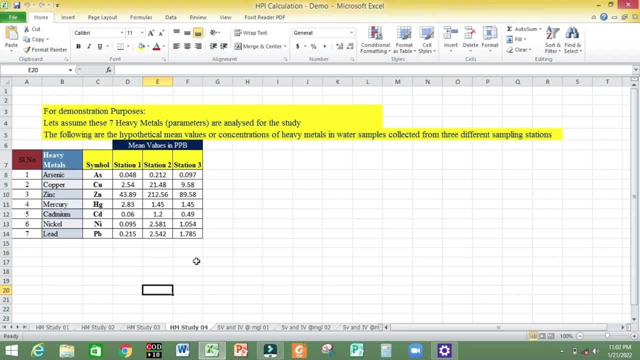 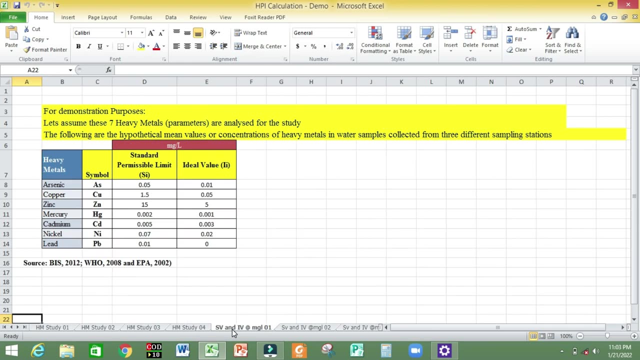 monitoring values and, as i said earlier, all analytical data should be in parts per billion or converted to parts per billion. now the next important data for calculation of hpi are standard permissible limit and the ideal values, or the si value and the ideal value. so now for different heavy metals that we analyze in our hypothetical study. these are the si value. 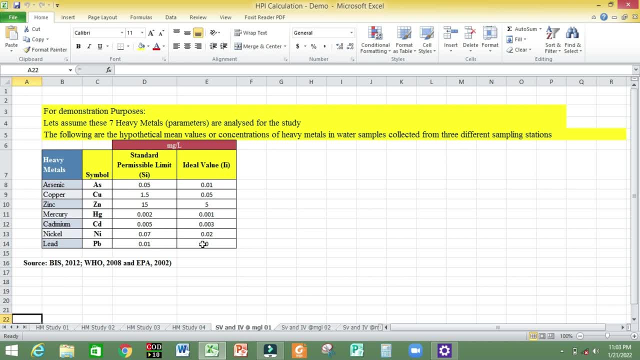 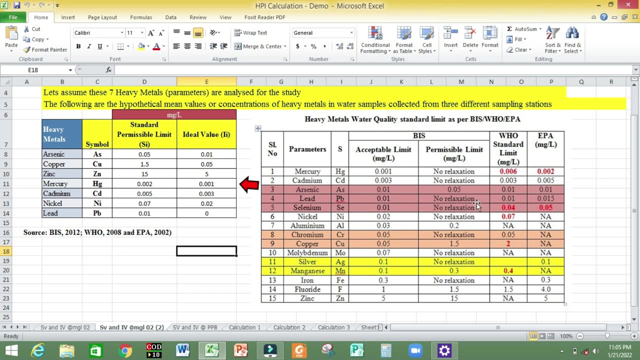 and these are the ideal values, which are in mg per liter. for your information and as a reminder, the si and ii values are obtained from this table, which in turn, contain the standard permissible limit for water samples for different heavy metals, as prescribed by who, epa and wis. okay, now these are the value for si. 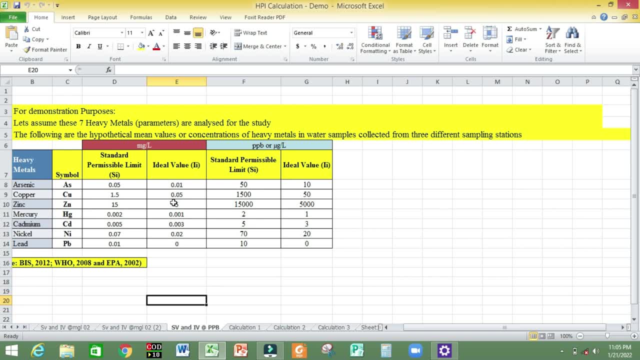 value. these are the ideal value. but this value, if you have to use it for hpi calculation, these values have to be converted into ppb. so si value, which is an mg per liter, if i convert it into ppb it will be 0.05. into 1000, you get 50.. 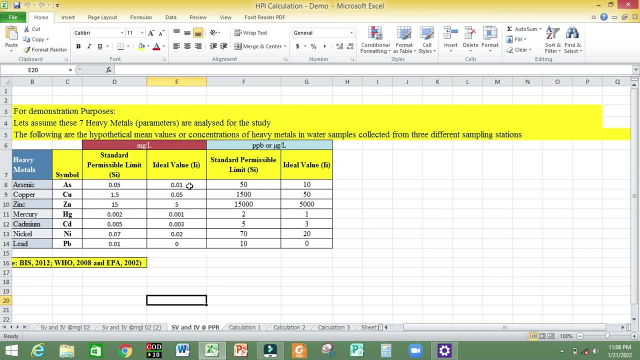 similarly ideal value, which is 0.01. if, if i convert it into ppb, i have to multiply it by 1000, so it'll be 10.. for 1.5, if i multiply by 1000, it will be 1500: 0.05 for couple idle value. 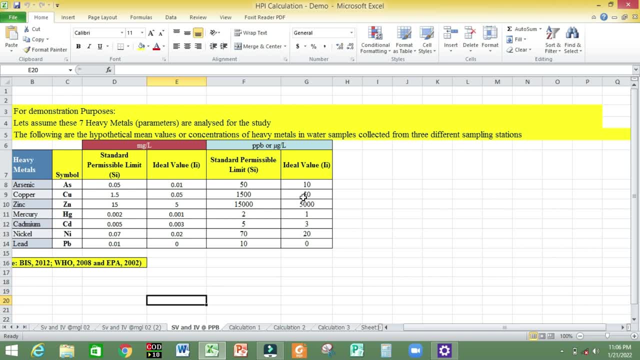 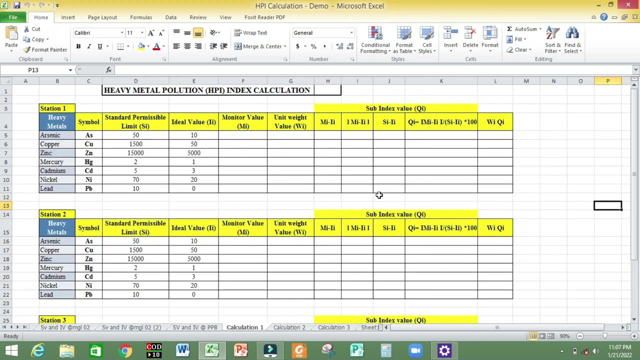 if i multiply by 1000, it will be equal to 50.. similarly, same way here: two, two for all: 5.015. this value you have to multiply by 1000, and now you'll get the si value and the ii value in ppb, because you're going to use it for calculation in ppp, not in mg per liter. okay, now for explaining. 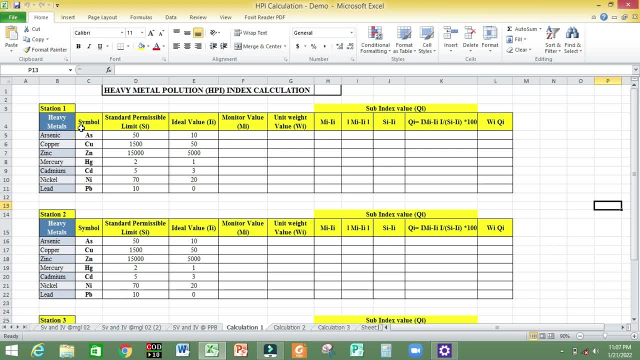 the heavy metal pollution index calculation procedure. please make sure you arrange this data in this format and then it will be easier for you to do the calculation, because calculation will be carried out station wise, station one, station two, station three and in station one these are the heavy metals analyzed and these are the standard permissible limit or the. 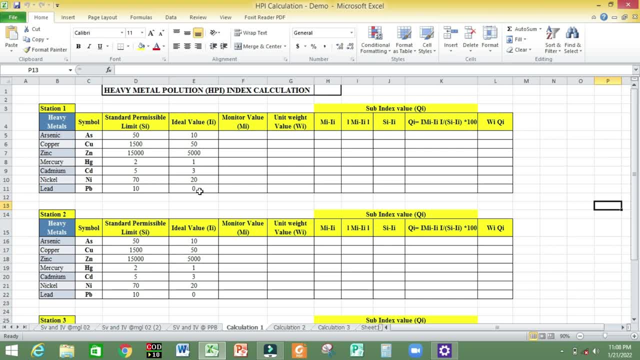 si value and the ideal value in ppb- now remember mi- is the monitor value or the value in ppb of this data, which is the in ppb we already have the limitee of the patient left side of the body, of the basic level and this isn't permanence lux, but it's the estimated amount. of things that we will do for calculating in this model. if you want to calculate plutôt out of this data, write down this and then sometimes you can do it in ppb and remember if you are längua re this webinar and then after warm up, you may already have to google dictionaries. 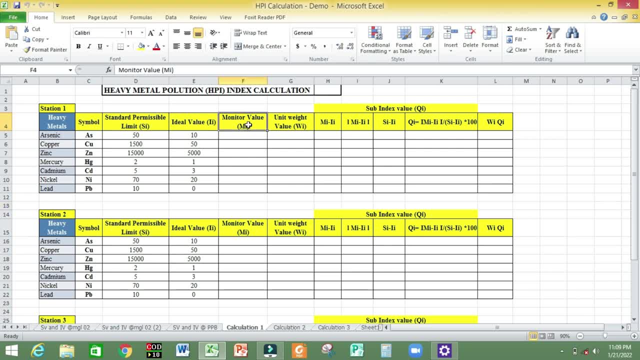 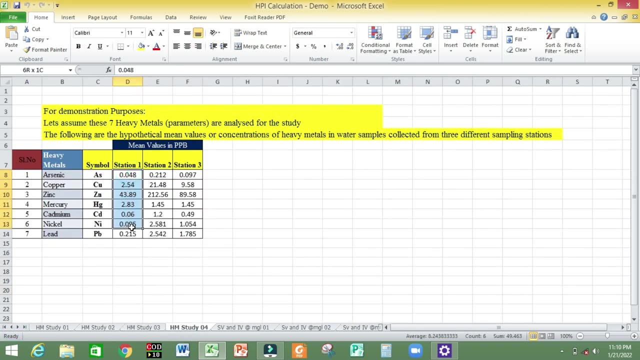 obtain after you analyze the water samples. let's now take the, the monitor value for station one. you have to go back to the sheet where the data is there. yeah, this one. what you have to do is just copy your station one data. okay, copy. okay, copy this data and then 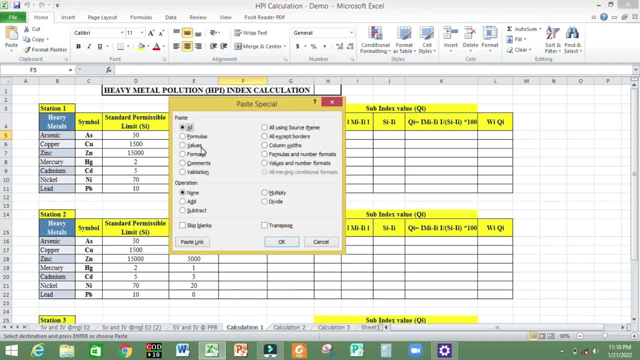 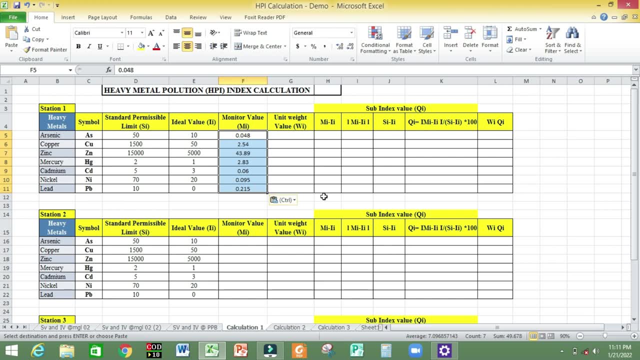 paste it here. be special. go create value- okay, this is your mean- or monitor value. now, what is wi? remember the formula. the formula for wi is k by si, so you just have to put equal sign. k is: remember the k value is 1 divided by si. what is si? why do you hear the si values this right for arsenic and turkey. you'll get this so. 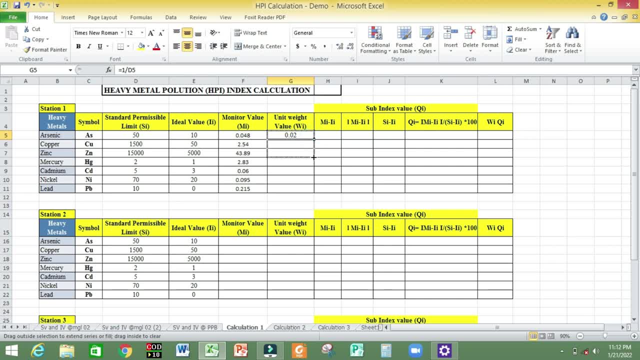 similarly, i do so. you just have to drag this. for the rest, you'll get the wi value. now here, mi minus ii. now for this column, mi, just put equal sign, mi, which is this: 0.048 minus ii minus ii. is this right, the ideal value? you'll get it at this. 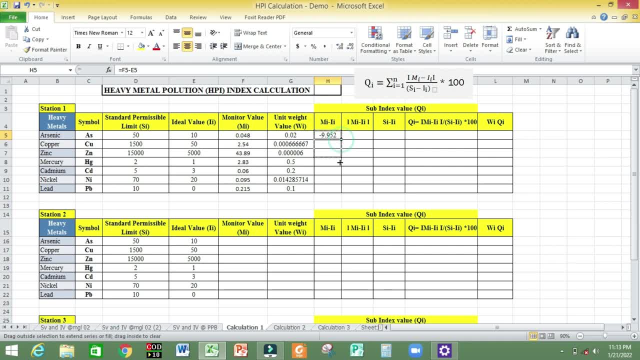 similarly you'll do for the other heavy metals. now you'll find that here there is a negative sign. remember i mentioned that whenever you have a modular sign, the negative sign will be ignored. because of the presence of the modulus sign, this value will be no longer minus nine point nine five two. it'll be. 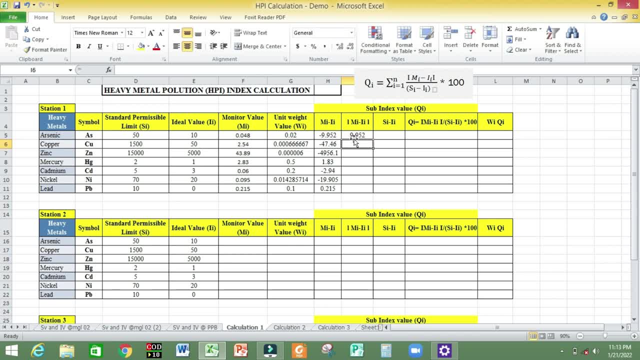 nine point nine, five, two. similarly, for the next cell it will be forty seven point four, six, four, nine, five, six point one, one point eight, three, two point nine, four, nineteen, ten point nine, zero, five, zero point two, one, five. okay, so you have entered all these and all these. so see, just cross check. 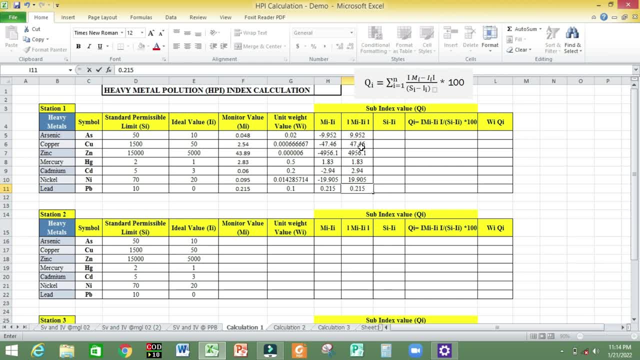 in case you you're mistyping or something like that. nothing else like it's fine, fine, fine, fine now. see, this is the purpose, where we have the modulus sign. now all the negative signs are ignored and now we all have positive values. now the next column for this: qi values: si minus ii. 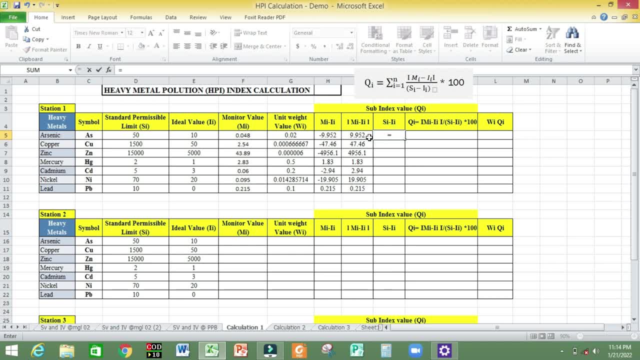 is equal to si. what is si, si? is this value right? 50 minus ii, minus ii is the ideal value for arsenic. so which is 10 will be 40. so similarly, since it's the same formula, you can apply for all heavy metals, you just have to drag once you have this value like this: next we'll calculate the. 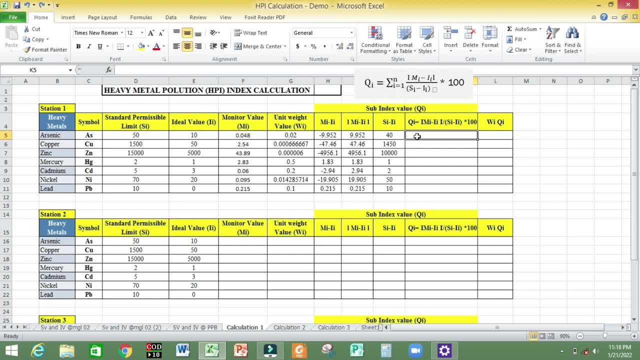 qi value. for qi value, it is equal to qi value. it is equal to mi minus ii. and within modulus, which is this: divided by si, by ii, which is 40, right into 100, enter, you get this much value for qi. so this is how you'll do for the other heavy metals. 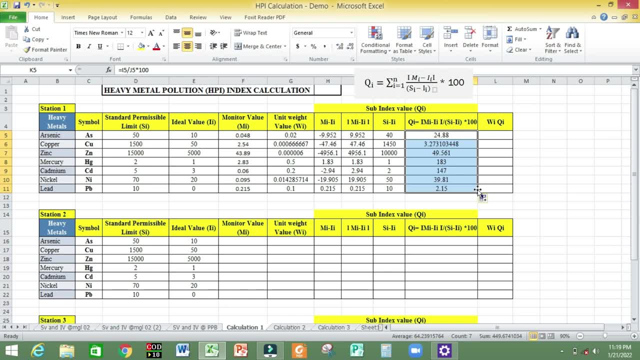 it's in the same formula, so you just have to drag it. now you have got this value. next, since you have got the qi value and wi value, so we'll get wi- qi value here. so just put equals to wi. what is w where is wi? wi is 0.02 into qi, value is 24.88. right, correct, now it's just the same. it's the same, can be. 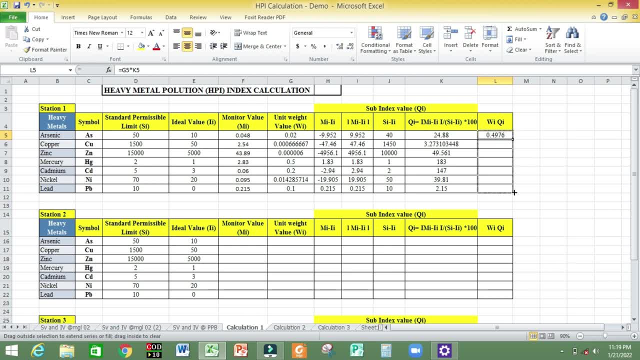 you just have to drag for the others, heavy metals, right now. once you have completed this stage- now you have completed for each and every single component of the hpi formula, now you have to calculate the final part, which is the numerator. the numerator is summation of wi into qi, just put. 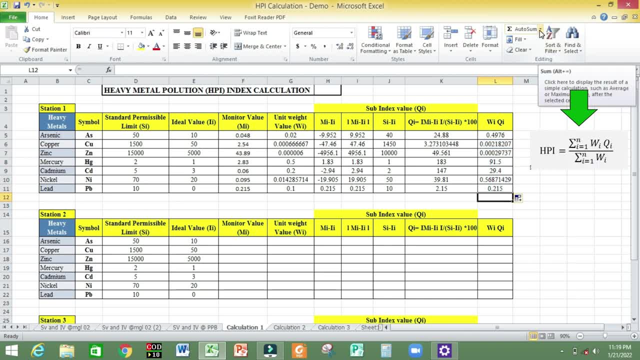 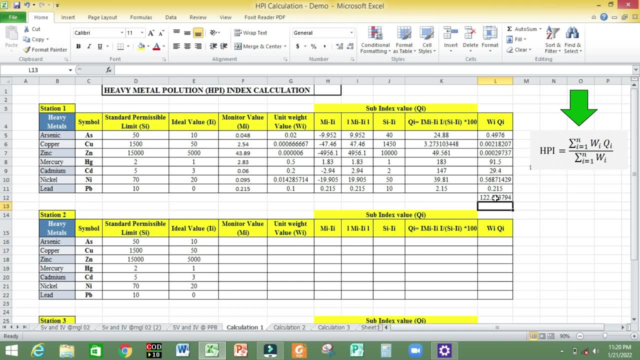 a click here, go to auto sum, click on sum and then enter. you'll get this much. this is the numerator with summation of w i, q, i, this value- right now the denominator is summation of w- i, so where's w i, the unit weight here? so, similarly, just click on this cell, go to auto sum, click on sum and click enter. so this: 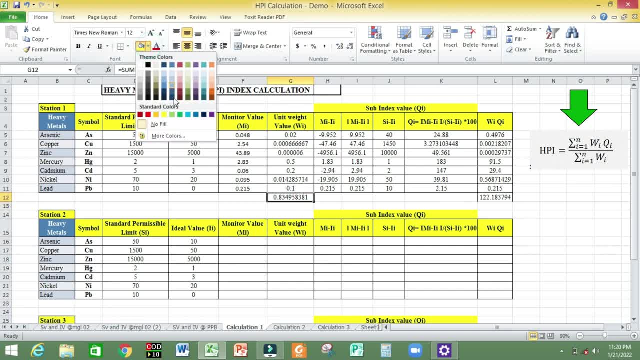 will be summation of. let's keep it in different, separate color. now. this will be the summation of w i. this is summation of w i, q i. so hpi formula is equal to summation of w i into q i, which is this divided by the summation of w i, which is this. so now, with this, you'll get this much. 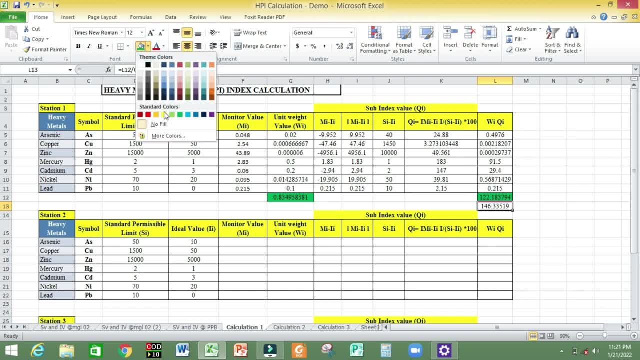 value. now let's put this inside the red color. okay, so like this. so now you will obtain the hpi value for sampling station one. okay, so now this is for all the different heavy metals. for station one will be 146.33 then, which means that, based on this calculation for sampling station one, we found: 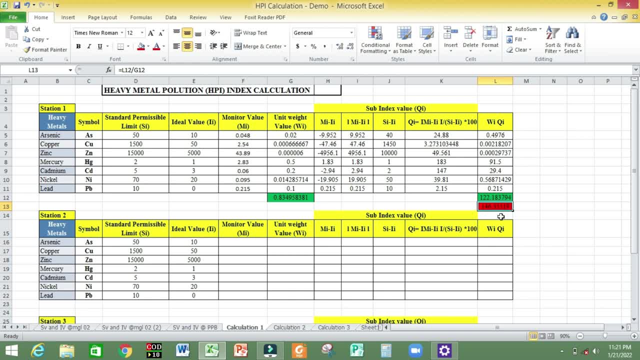 that the hpi value is greater than 100, which means that the water sample is polluted with heavy metals. simple as that. okay, now, if you want to calculate the hpi value for each heavy metals within the same table, just have to add the summation of wi here. so what is the wi value? zero point. 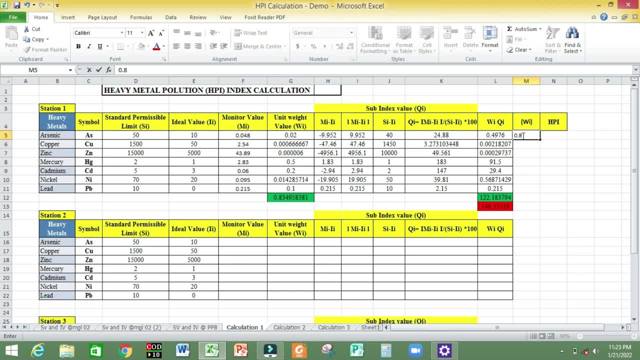 zero point eight, three, four, nine, five, eight, three, eight one. okay, so the wi value is this much right. just put it the same to all the different heavy metals. now you have the wi value here. now for hpi value for each of these heavy metals would be, starting with arsenic, wiqi value for arsenic is 0.4976, right. 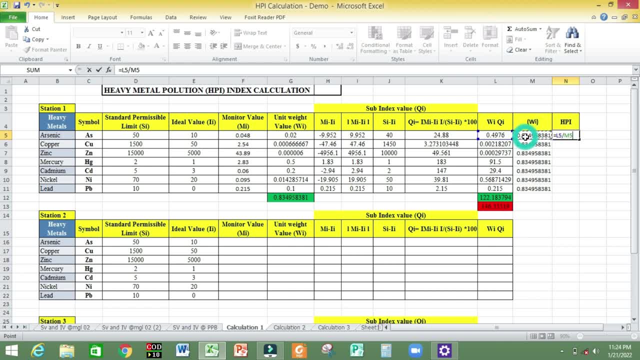 then you divide it by wi value, which is this much so this will give you the hpi value of arsenic. similarly, you can just drag for the others which you will find by this way. and now from here, from this calculation, you can also find out which heavy metals. that, has been analyzed, contributes to the increase in. 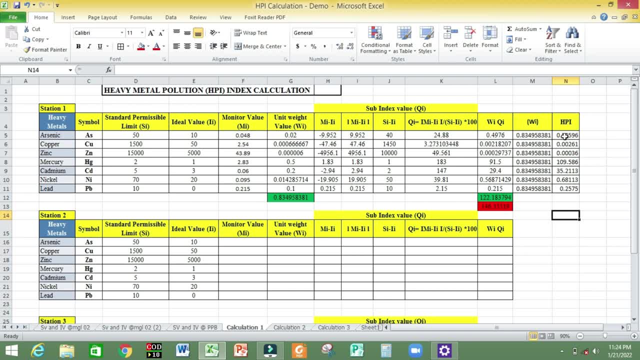 hpi value for station one. from here you'll find all these seven parameters except mercury. mercury parameters are below 100, so which means that the main causes for the heavy metal pollution in the water sample in station one, the main contribution, is mercury. okay, so similarly in 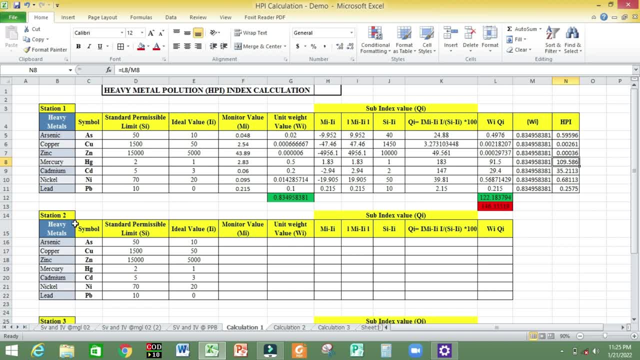 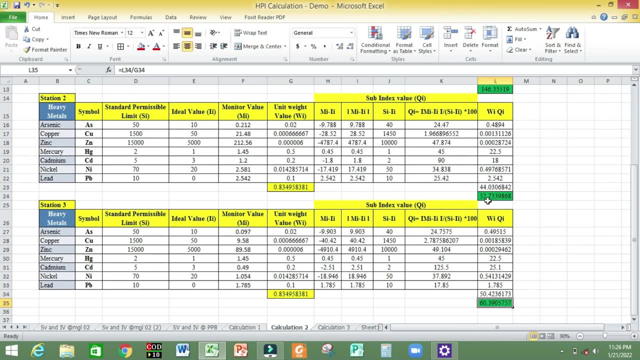 the same way you'll do the calculation for station two and station three and, in order not to waste time, i've already calculated it. so for c for station two, the hpi value is 52.73 and the hpi value for station three is 60.39. so in both the case- station two and station three- we found that 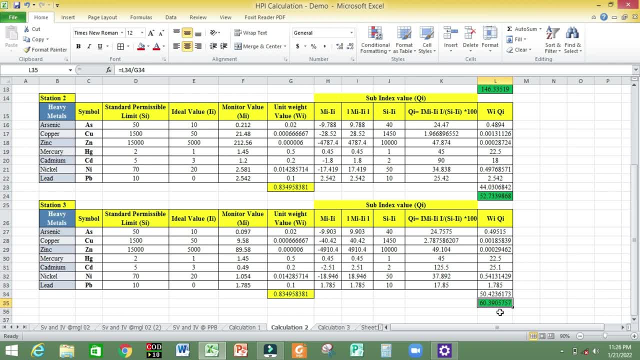 the hpi value is less than 100, which means that the water sample is safe and free from heavy metals pollution. and in the same way, if i want to calculate the, the, the hpi value for each heavy metals, same way, i just take the wiqi value and the wi value, then these are the values we'll get. the. 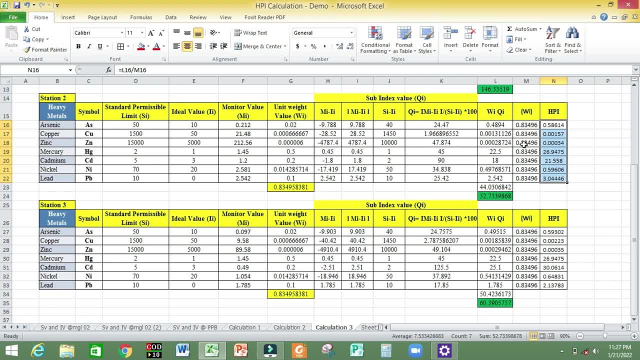 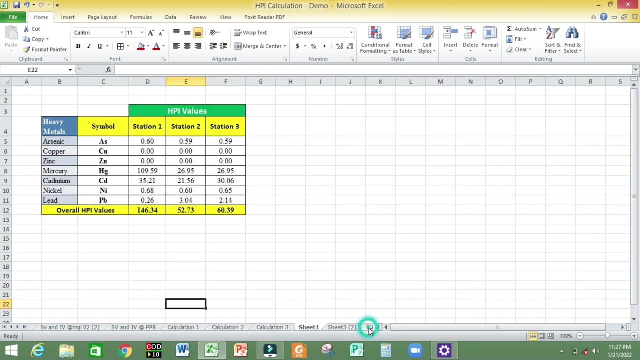 hpi value for each of the heavy metals. for station two, now you see that all the values are less than, which means that the water is free from heavy metal pollution. similarly, for that of station three, all the values are below 100. so now, from here, if i put it, all this data together, then i'll get the value as this. 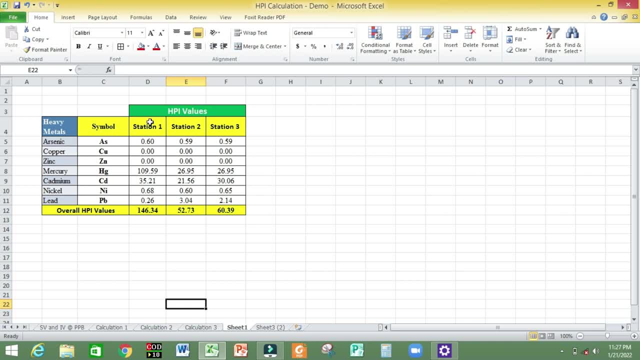 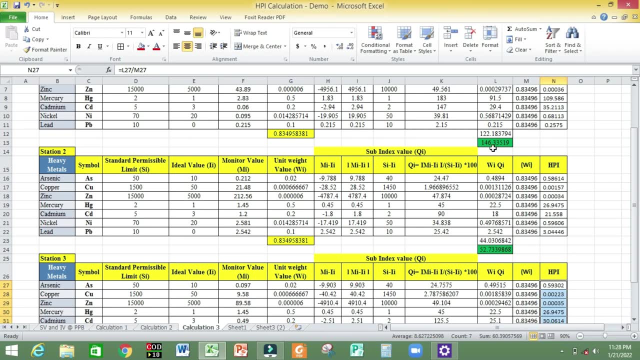 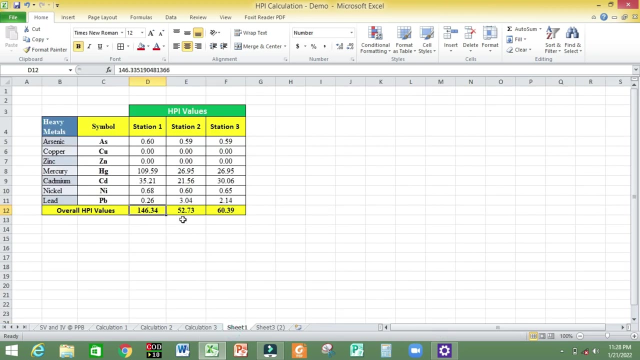 the computed hpi value for different station are: station one, if i compile it from there, it is 146, see 146.35, and for station two it's 52.73 and for station three is 60.39. so see the hpi. overall hpi value for station one, two and three are obtained and from here we can conclude that